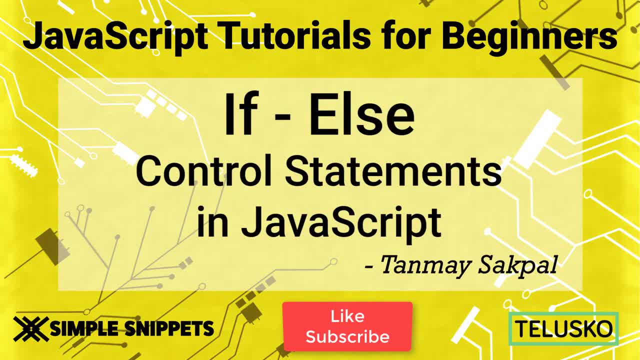 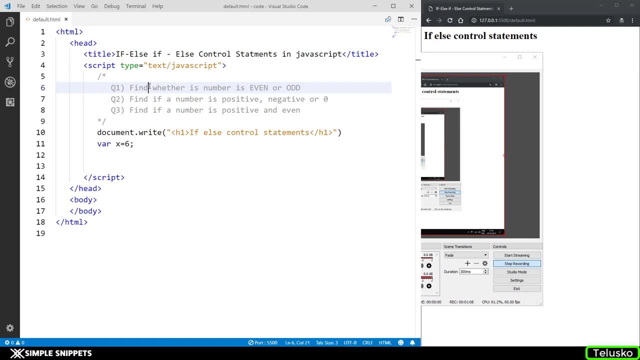 Hey, what's going on, guys? Tanmay here for telesco learnings and in this video tutorial we're going to be taking a practical approach and understand the- if else control statements in JavaScript. So in the previous video we saw what are control statements and we saw the different types of control statements. 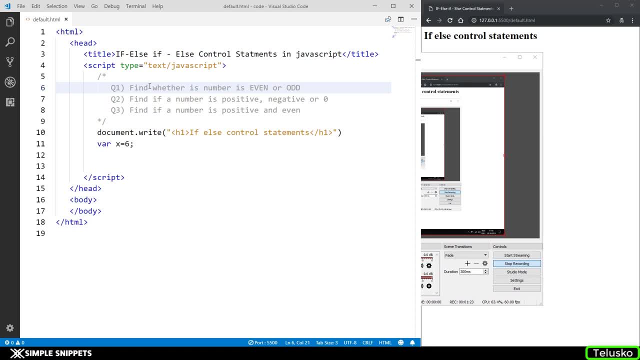 and we took a theoretical approach. So if you have missed that video, you can check it out in this playlist. But in this tutorial we're going to be seeing three different programs based on- if else, control- statements. So let's just quickly get into the topic and open up. 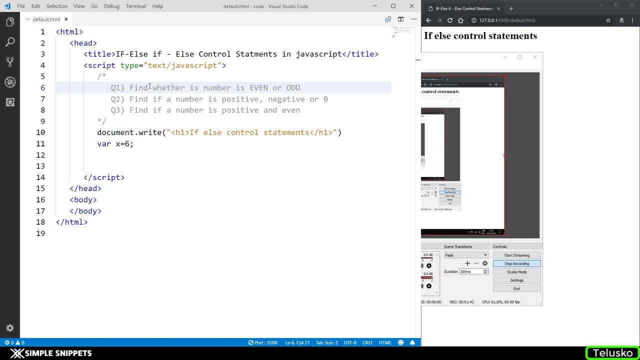 your visual studio code or any text editor that you're using And, as you can see, I've already opened up mine and I also have opened up the Chrome browser, and we are live. So anything that I change over here is immediately visible in the output. So that's that, live. 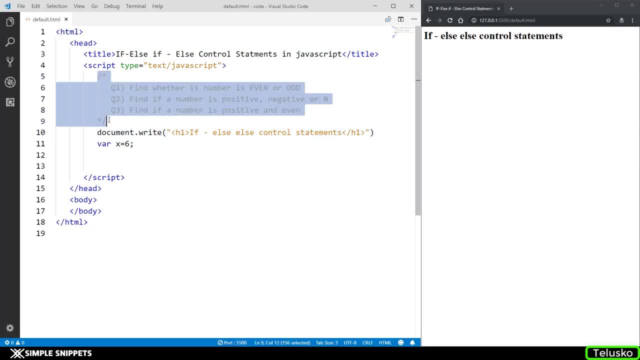 server plugin that is active And as you can see on the screen. these are the three different questions that we are going to be writing program for, So let me just read it out quickly. So the first question is find whether a number is even or odd. Second is find if a number is positive, negative or zero. And the third 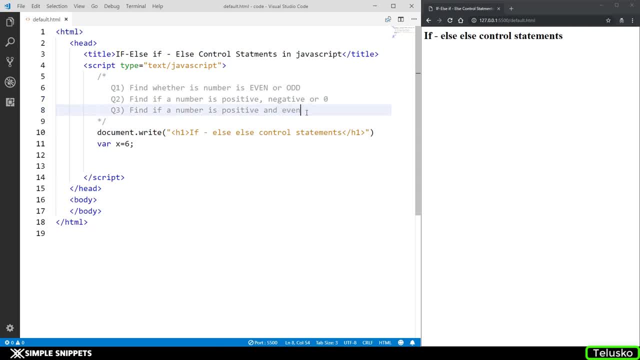 one is: find if a number is positive and even. So, these are three different variants of if else control statements, and we'll see the different types. So let's start off with the first one, that is, find whether a number is even or odd. Okay, so, as you can see on this, 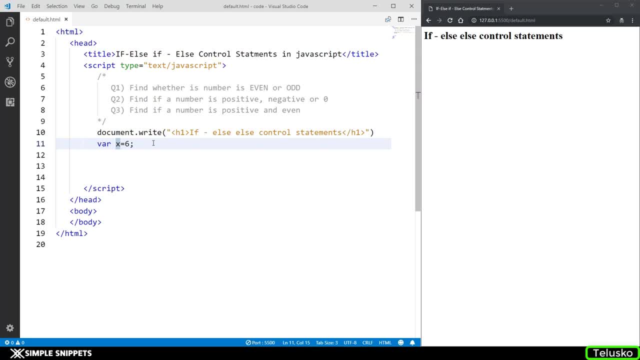 line, I have created a variable where x equals to six. Now, for simplicity purpose, I'm not taking values from user, because we still have to understand what is Dom manipulations and how to take values from textbox. We still haven't reached that level, So, as of now, I'm just hard coding the values that. 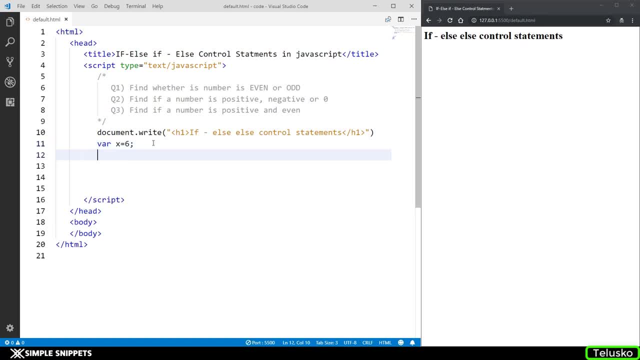 is, I'm directly giving values in the code. So I have a variable x who's storing a value of six over here, as you can see. And now we're going to do if else control statements. So this if else control statements helps us determine a particular condition. So what? 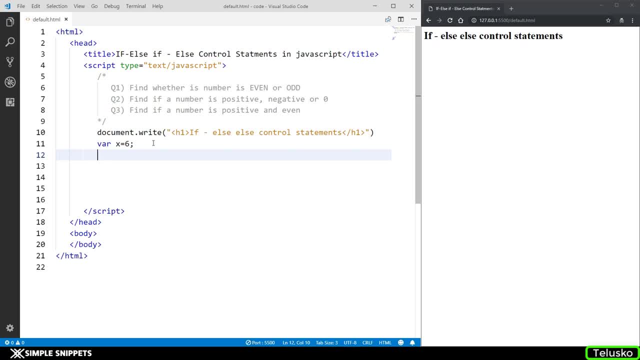 is the condition in question. number one: we have to find out whether the number is even or odd. So this is how the syntax goes. You have to write: if that's the syntax, So that's the keyword, and then opening and closing round brackets And inside that you have to. 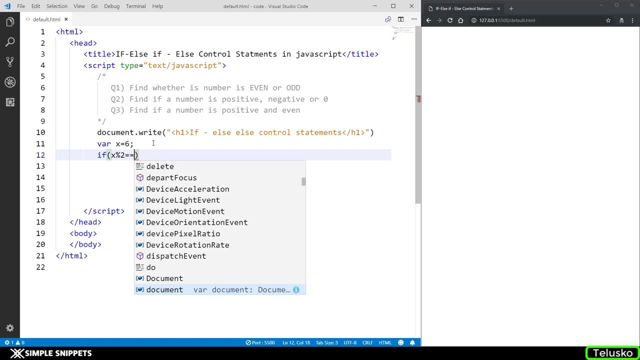 see x mod two equal, equal to zero, then opening and closing curly braces. So this is that if block, and I'll explain to you what this condition is. So what we're doing is we're checking whether the modulus operation performed with the variable x is giving us a result. 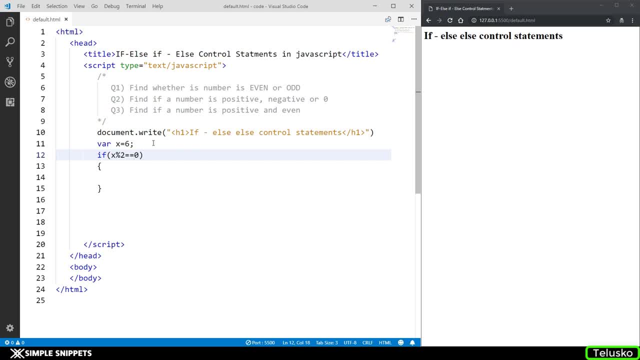 of zero. Now we know that even numbers, when divided by two, will always give us the result of zero, right, That is, the remainder is going to be zero. let's say six, Eight, 10,, 12,, 1620, any number that is. even if we divide by two, the remainder is going. 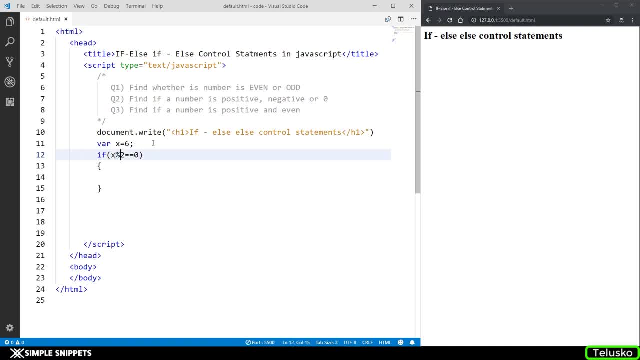 to be zero. Now the modulus operator. so this is that modulus sign- always gives us the remainder. So that is what we're checking. So we're seeing if this variable x is taken and if you perform a modulus operation with two and if it results in zero, obviously it is going to be even. 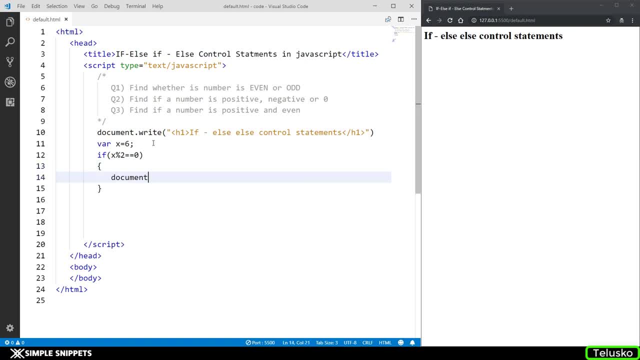 number right. So here what I'm going to write is document dot right In the opening and closing round brackets. the text that I'm going to write is even number. So in fact, as you can see immediately, the output is also being shown over here. Let. 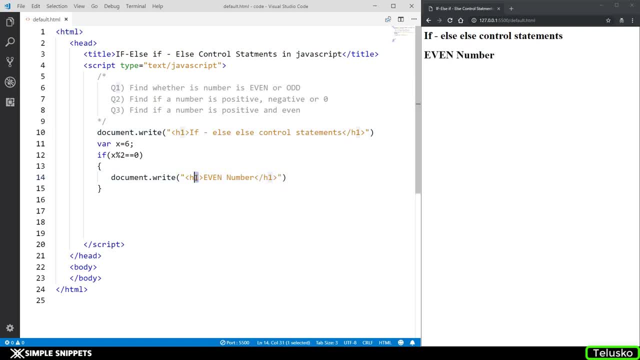 me just put it in H1 tag. In fact, I'll do it in H3.. And the reason why immediately we got even number as output is because, yes, we can see that this variable is even And that's why this, if block got executed. So what if this variable was not even? let me 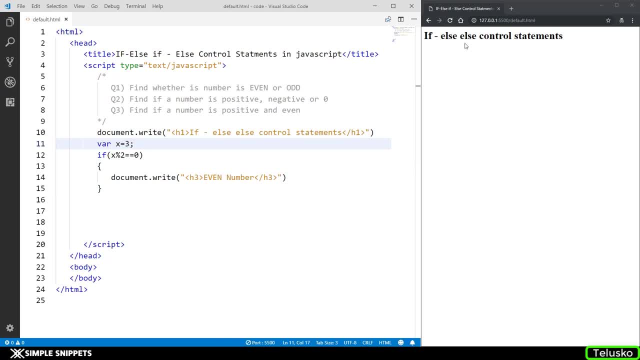 just change it to three, So they will go. you cannot see any output now. But we also have to find out for the odd side right, We also find need to find out whether the number is odd also. So in this case, simply I can see else, I'm just. 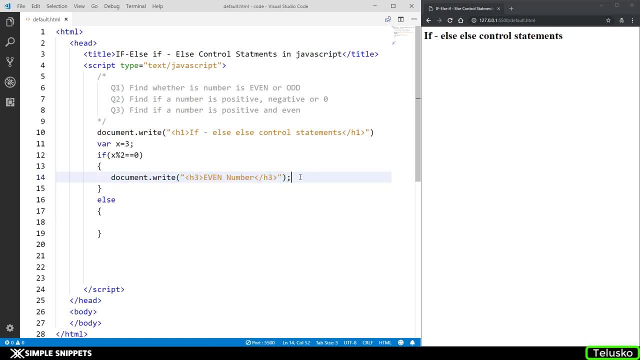 going to copy this entire statement. I forgot to give a semi colon And here I'm going to see odd number. So now you can see we are getting the output of odd number over here. If I change this value to two again, we'll get even number. So this is the if else control. 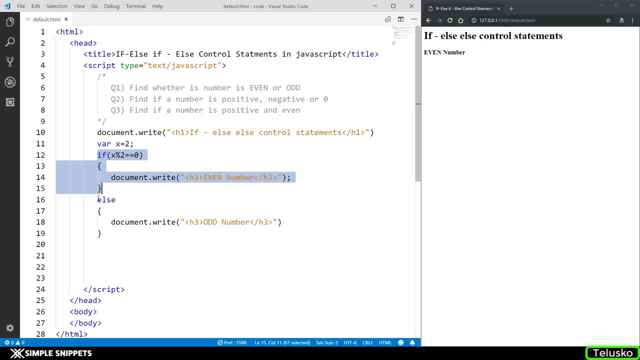 statements. So either the if block is going to be executed or the else block is going to be executed, depending upon what the condition is. Now note that you can always exclude else block, so we don't need to have it. So if you have only one condition, to check for that. 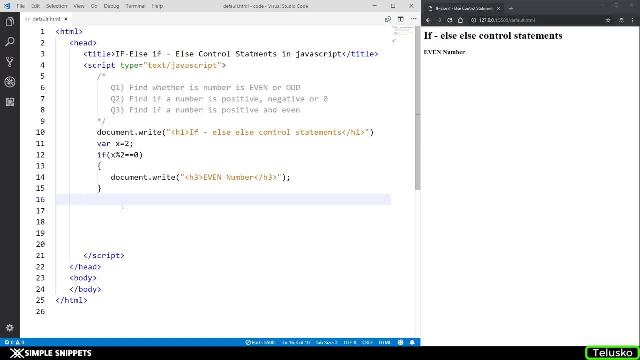 is only. if you want to check for even numbers, then you can do it in a block, itself right. But if you are checking for multiple conditions, then you can have if, else if and else. so that else if part we'll see in a minute. but you cannot have an else block in without a. 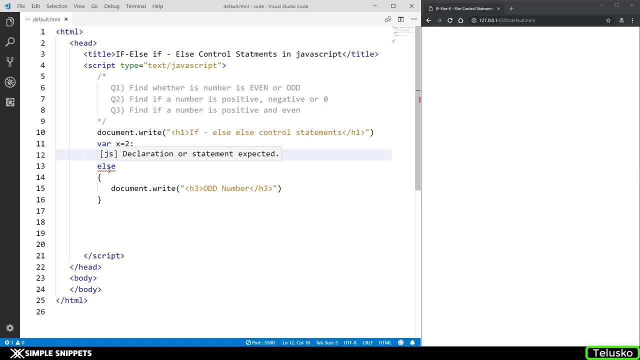 block. Okay, so that is not valid. You can see that immediately. we're getting an error. Okay, so this was the first program. Now let's actually get to the second program quickly. and it's just a simple modification in the first program itself. So the second. 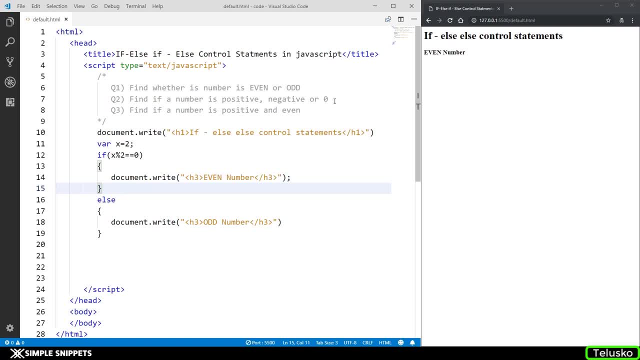 program is saying is we need to find out whether number is positive, negative or zero. So now let's see our variable: is x equals to two? as of now, What do you have to check in the if block? We'll see. if x greater than zero, I'm going to see it as a positive number. 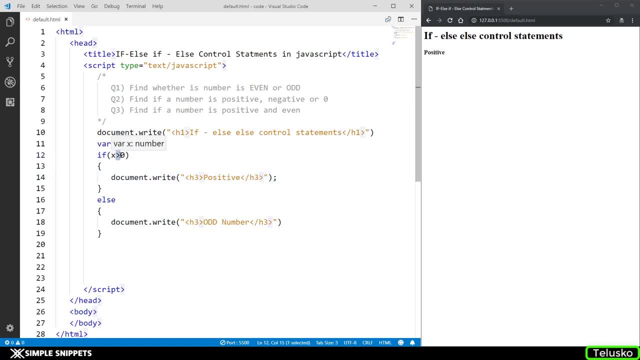 So these are those comparison operators we've talked about in the operators video Right. So these are the comparison operators which help us in performing the comparison. Now we also have to check for negative numbers, So I'm going to say else. if again opening. 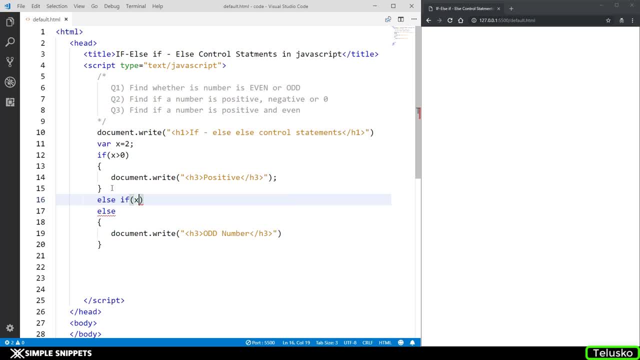 and closing round brackets. So this is how else, if block goes, I'm going to say x less than zero And inside this I'm going to write negative. So if x value is less than zero, it's going to be negative. Let's change the value over here. I'm going to say minus one. 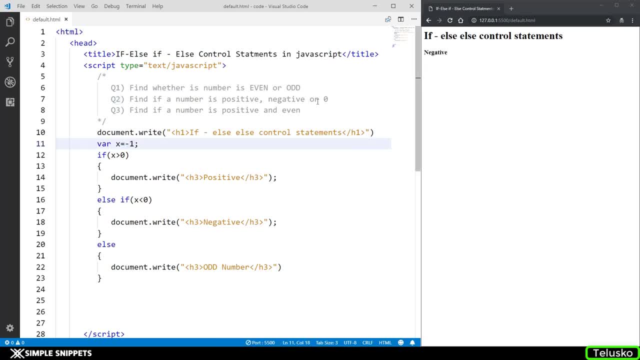 and you can say immediately: We got the value of negative. So, lastly, we also have to check for zero, right? So this is where the last else block can be used. I'm going to say number is neither positive nor negative. So if I make the x value as zero, let's see what we get. So there you. 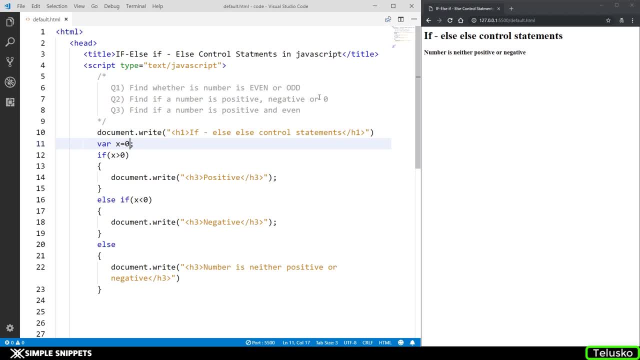 go we've got. the output number is neither positive nor negative. So here we had three different conditions, that we used three different blocks. we used if block, we used else if block and we also used else block. So this is how you use else if block. 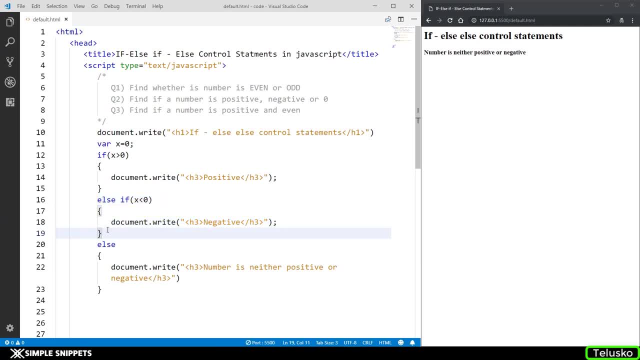 Now you can have n number of conditions and then just the else if blocks will be increased, right? So if you want to check for one more condition, you just need to add one more else if block. So this was program number two. let's quickly jump to program number three. 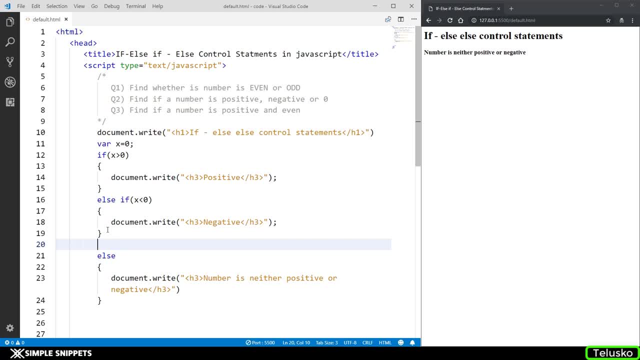 that is, find if a number is positive. and even So, we have two conditions, but they are linked with each other, with the and clause, which means that we need to check a number which is positive as well as even okay, and not just a positive number. So let's see how. 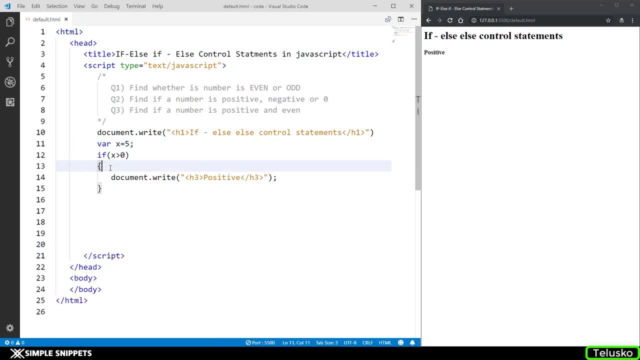 that goes. So let's say our number is five. So in the if block what I can do is I can have nested if else blocks, which means first I can check whether the number is positive. So this condition: six for that right. So if x greater than 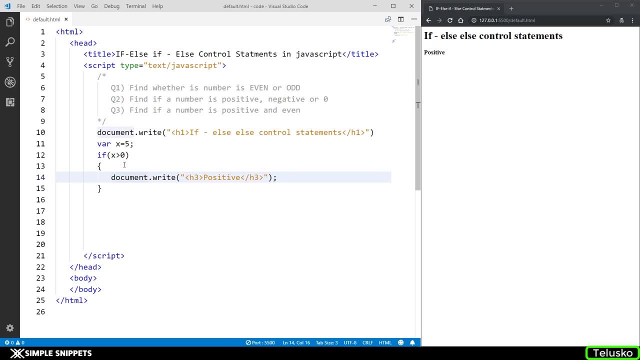 zero, which means that it is going to be a positive number. but I also need to check for even number eight. So inside this if block, I can see if x mod two equal, equal to zero, which means that it is also even number, And I can again print. 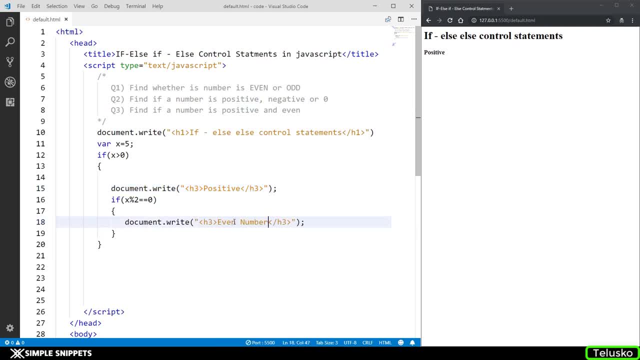 Even number And inside the bigger. if that is this if block, this if block, I can also have else block. So this else block will be for this inner if block. Okay, so here I can see number is positive, But it is odd, Correct, right, Because you can see our number is positive. 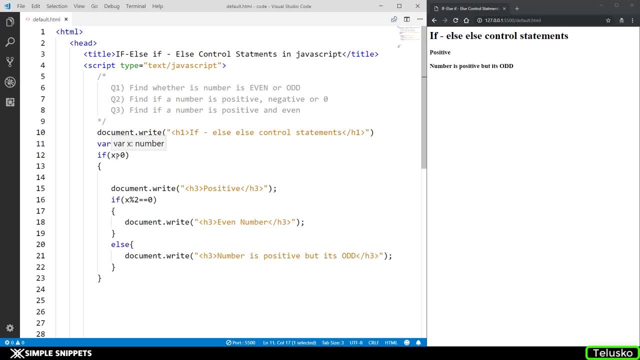 but it is odd. So first time checking whether the number is positive or not In this larger if, since it is positive, this internal block is executed, otherwise it would be excluded. So inside this first time printing positive: yes, we have our positive number. 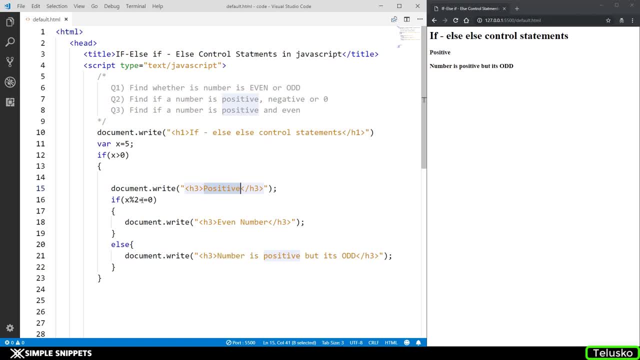 but we are checking for the next condition, which is if x mod two equal equal to zero, which means, is it an even number or not? If not, then the internal else block is going to be executed and it is going to say: number is positive. but it is odd Now for this outer. 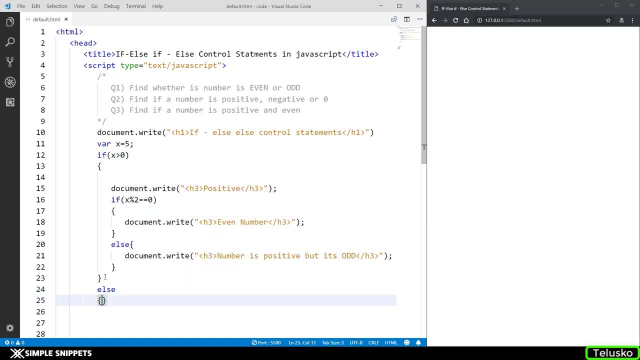 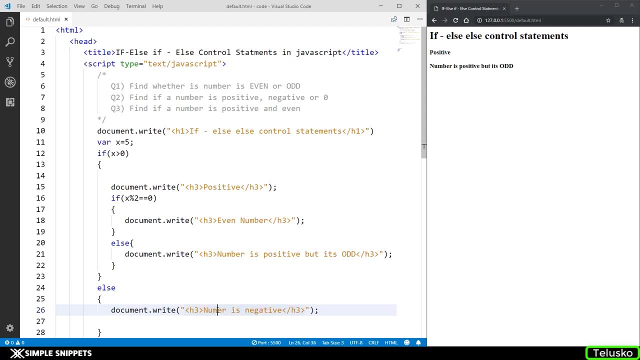 if I can also have else block When I can say number is negative. So if I had minus five or you're directly, we would have got number is negative. So I hope you're getting how to use, if else, if nLs, control statements and you can see that. 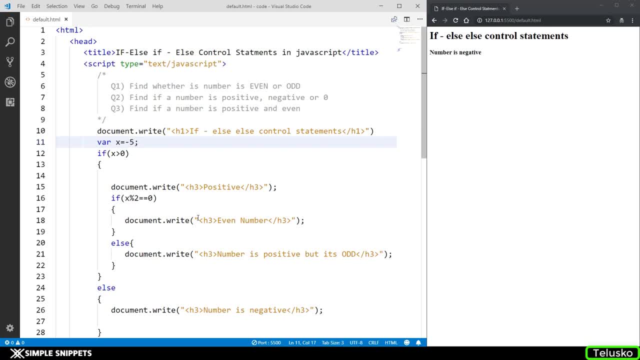 we saw three different vagrants and three different versions of how you can use them. Now one last variation that you could have done in the last program- that is question number three- is: instead of using nested, if else we can have both conditions in the first. 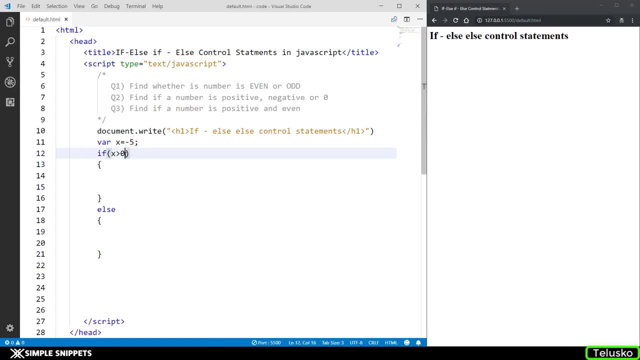 itself. So let me just show you how that works. So this is where we can use the logical operators, and the logical operator to be used over here is and because we need to find if the number is positive and even right. So first condition is going to check for x greater than zero.